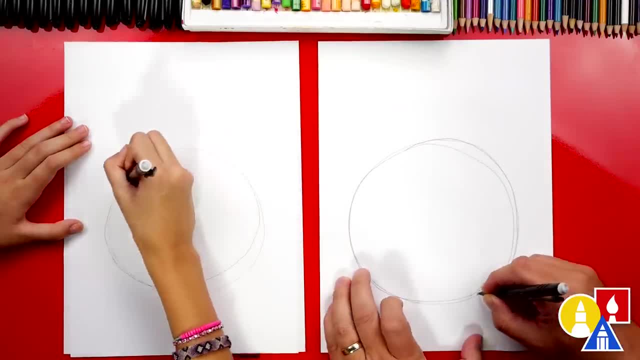 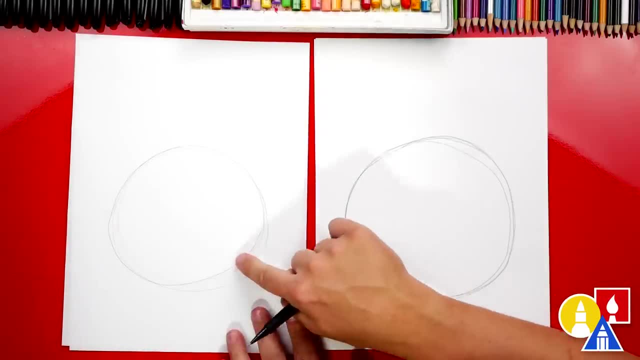 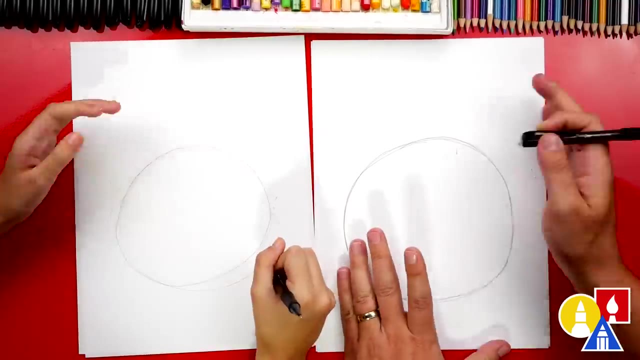 easier to erase at the very end And you can go back over it until you get the shape just the way you want it. And then, if you have extra lines, you can erase those so that you don't get confused with which line you want to keep. Remember to pause the video if you need extra. 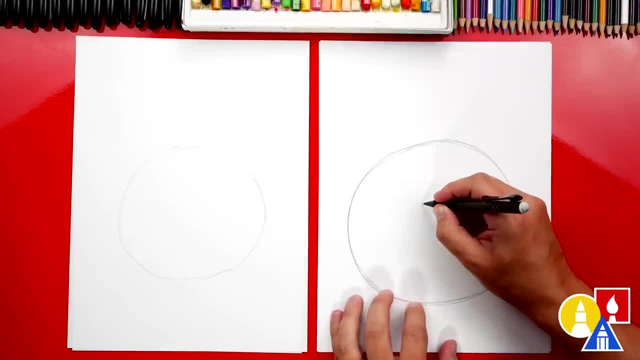 time. Now let's draw the inside of our donut. I'm going to draw another circle that's smaller and that's going to be the inside of our donut, And then I'm going to draw another circle that's smaller and that's going to be the inside of our donut, And then I'm going to draw another circle. 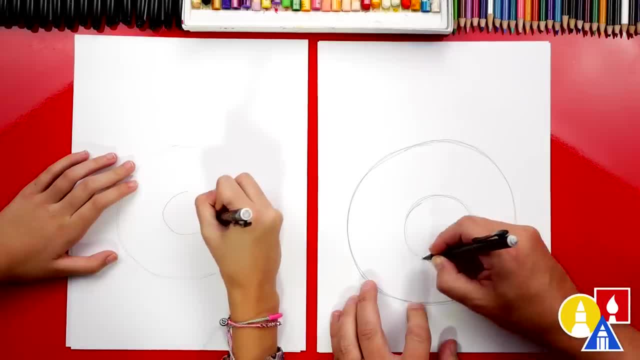 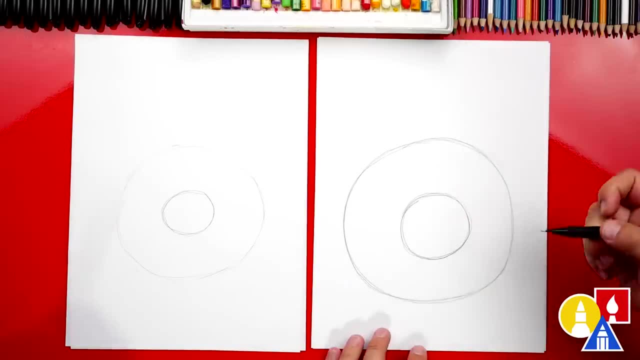 in the center and about that size. Go back over it. I'm pressing hard but you can press softly so it's easier to erase. We did it. We finished drawing the general shape of our donut. Let's switch to our marker next. And now we can add all of the details to our unicorn donut or turn it. 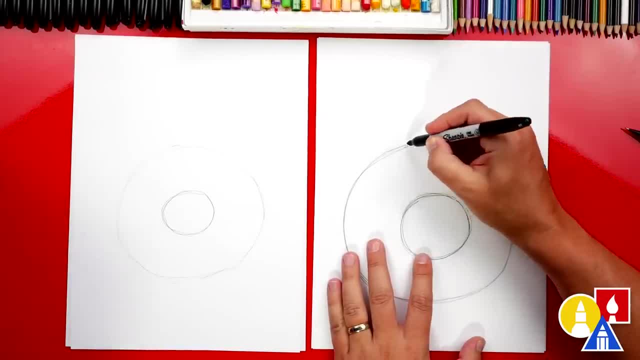 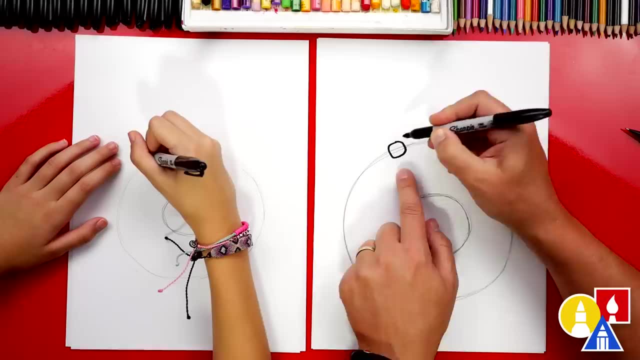 into a unicorn donut. Let's first start by drawing a bow. I'm going to draw right here. I'm going to draw the center of the bow. I'll cut it. You could draw a circle or kind of a square shape. 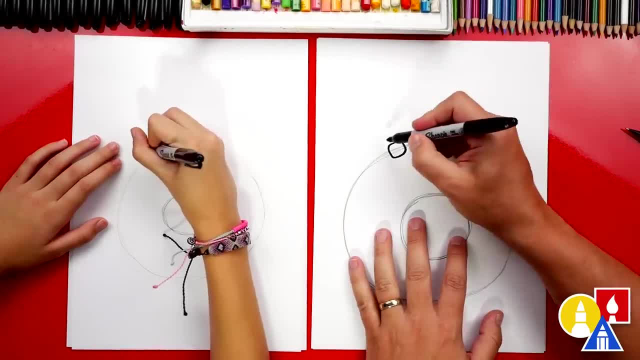 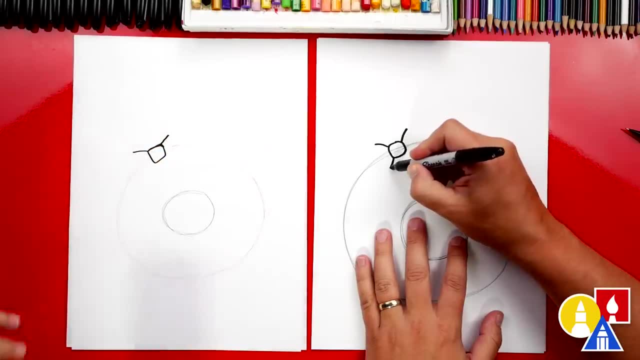 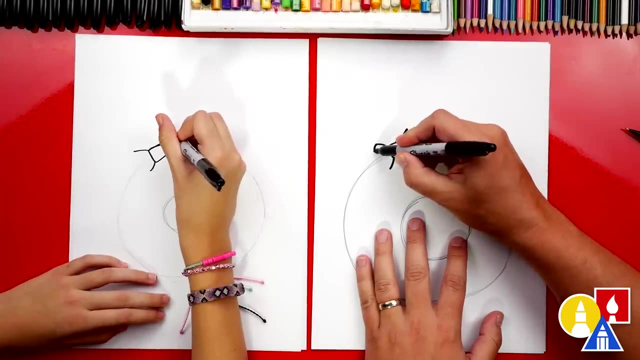 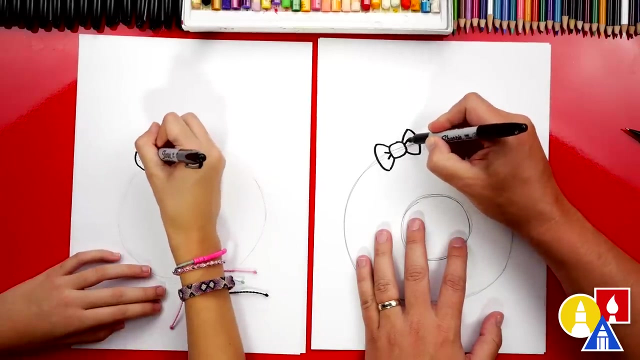 Then let's draw a diagonal line coming out of the left and also the right, And then we could also draw a diagonal line coming out on the bottom too. Then let's connect the top down to the bottom on the left and also on the right. We could also add two little wrinkle lines on the inside. Now let's draw. 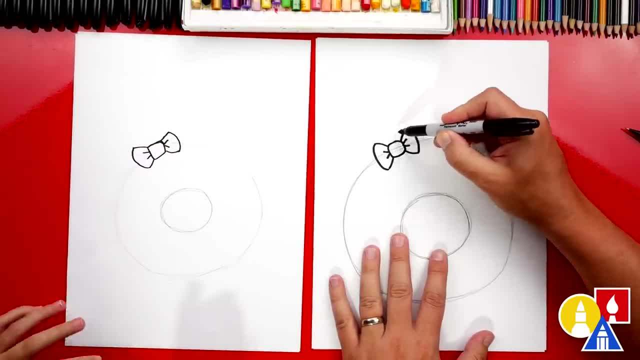 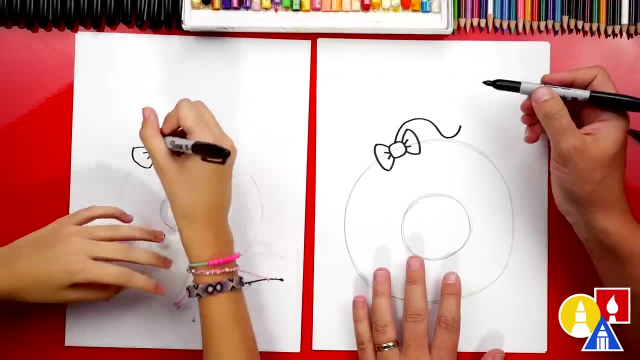 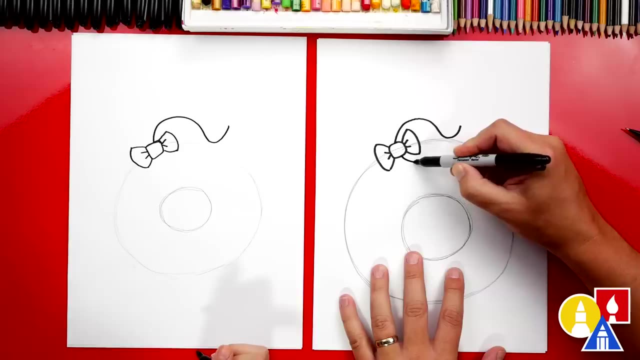 our donut's hair. Let's start on top of the bow. right here I'm going to draw an pair difficult come up Down and then back up. Then right here we could draw the bottom of the hair, coming down across, and then connect over here. 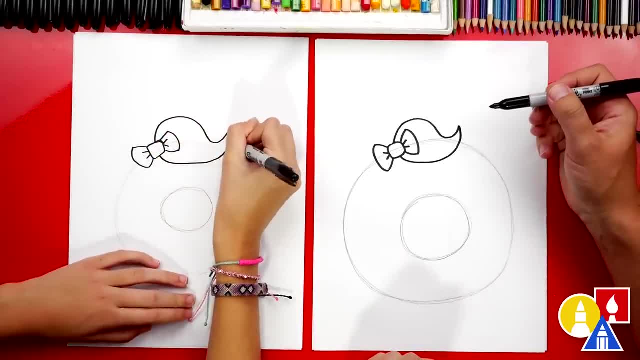 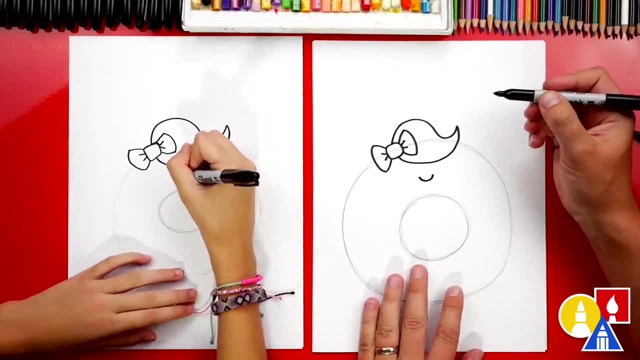 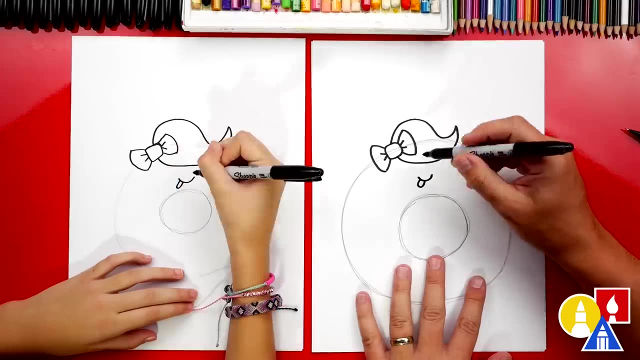 to this side. Let's add the funny face next. I'm going to draw a cute little smile right here underneath the hair, and we could also draw a little tongue sticking out to the side, if you want. but you could change your face too and add different details. I'm gonna draw. 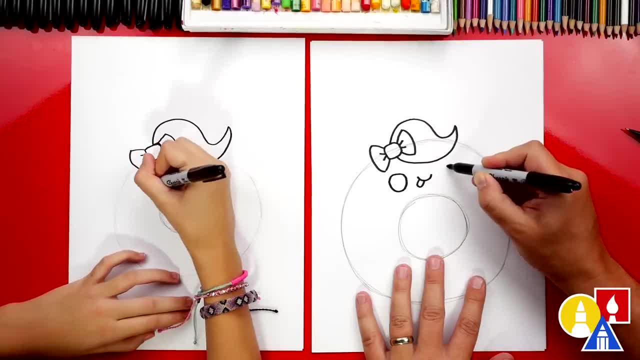 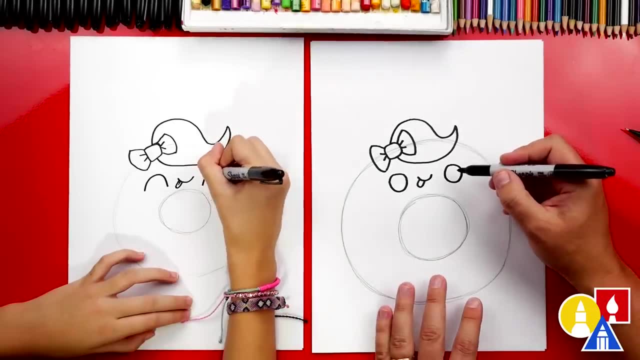 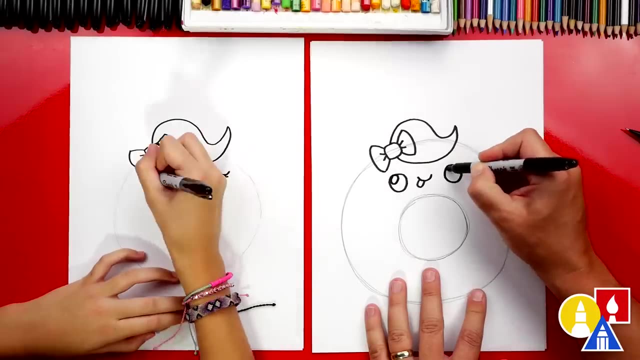 a circle for the left eye and also the same size circle for the right eye. you could change it so that maybe one eye is winking or closed where both of them are closed. I like that. yeah, we should add. I'm gonna add a highlight to each eye. 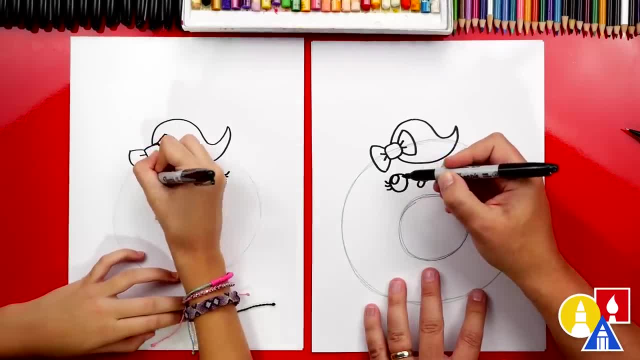 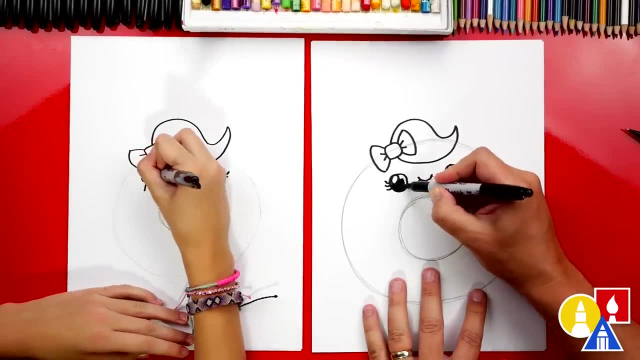 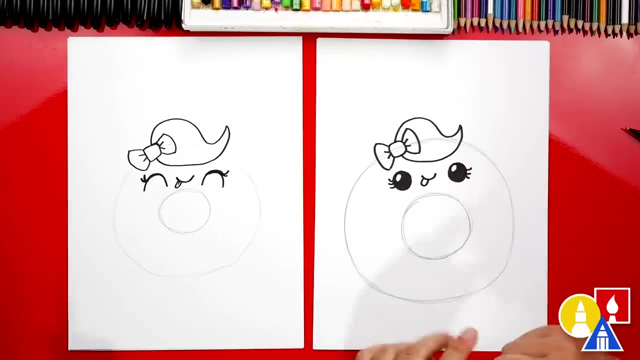 and then also eyelashes. like your eyelashes too. I like that your eyelashes are different. I'm gonna color in the big circle, but leave the little circle white. remember to pause the video if you need extra time. now let's switch back to our pencil- well, actually, the eraser part of our pencil. this part we're gonna fast. 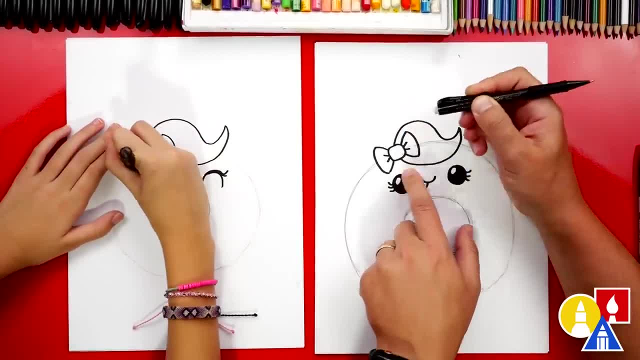 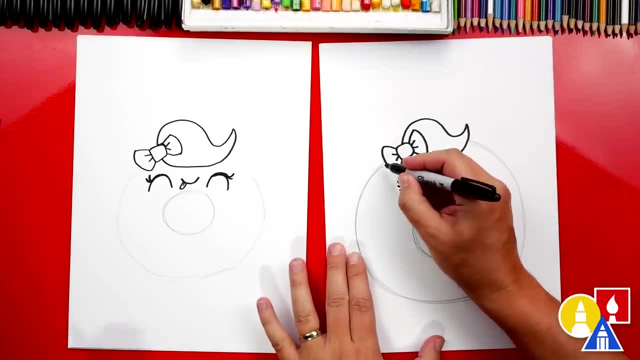 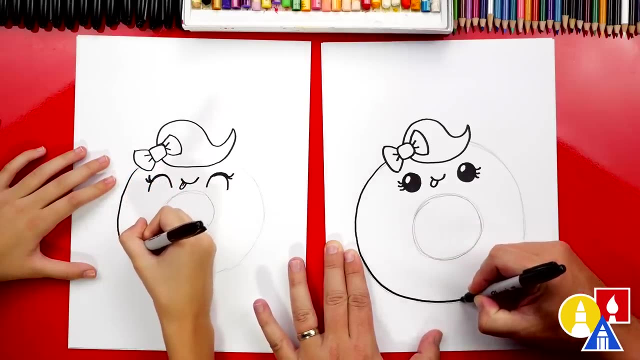 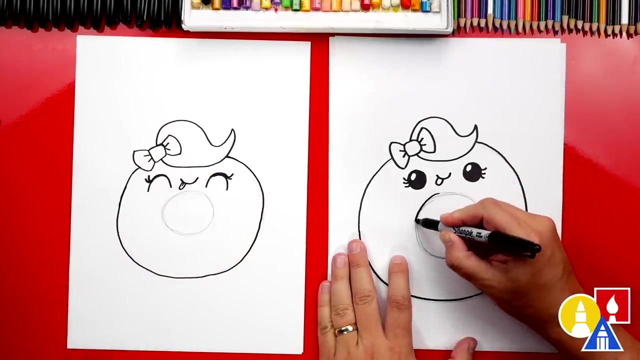 forward, but you can pause the video and take time to erase the guidelines going through the bow and also the hair. let's switch back to our marker and trace over the outside guidelines of the pencil for the circle stead. let's also trace over the inside circle, right on top of the pencil lines. 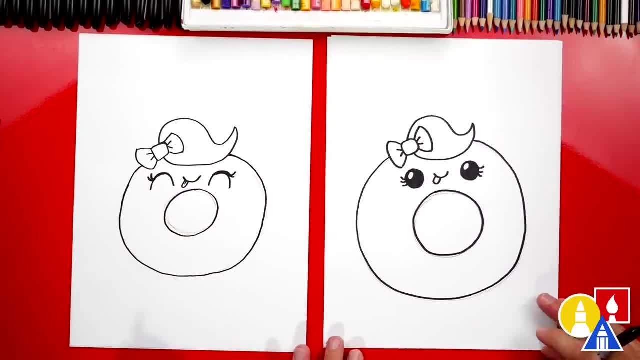 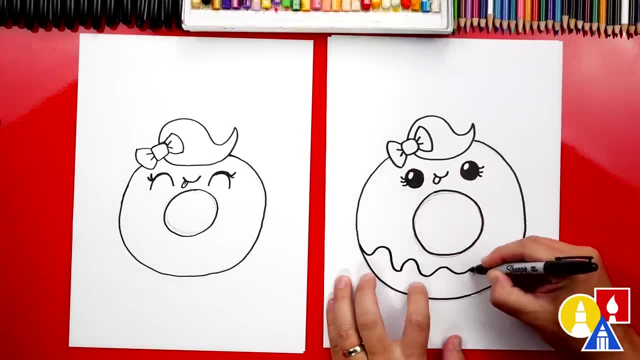 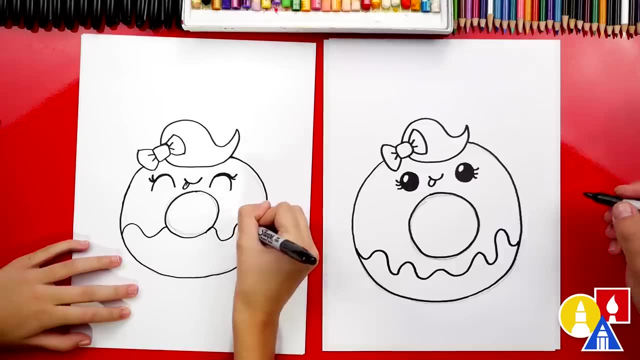 get shopping. what's our doughnut missing? frosting, frosting. let's draw it dripping down the bottom. I'm going to draw a wavy, wiggly line going across the bottom of the donut. Oh, I like that you connected to the center. 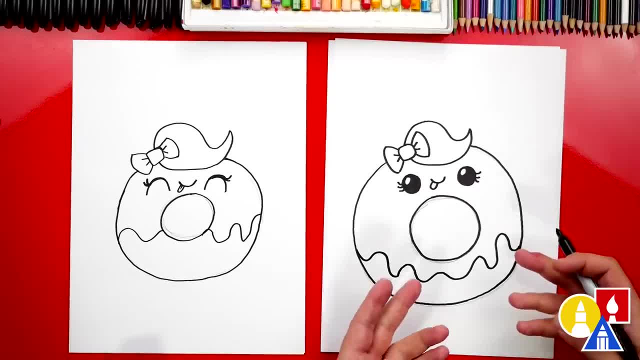 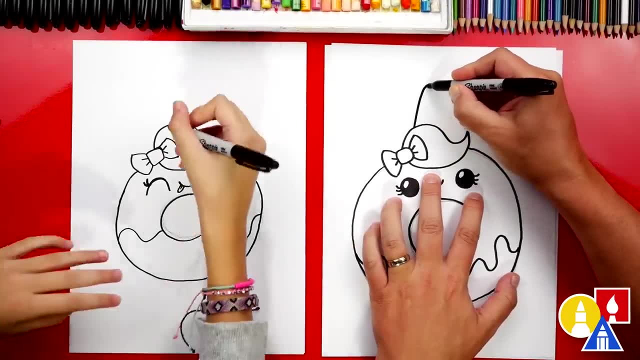 That's cool. What should we add next? The horn- Yeah, it just looks like a cute donut With hair. Yeah, with hair, Let's turn it into a unicorn donut. We're going to draw an upside down V, but at the very top, look, I drew kind of a curve so that it's not a sharp horn. 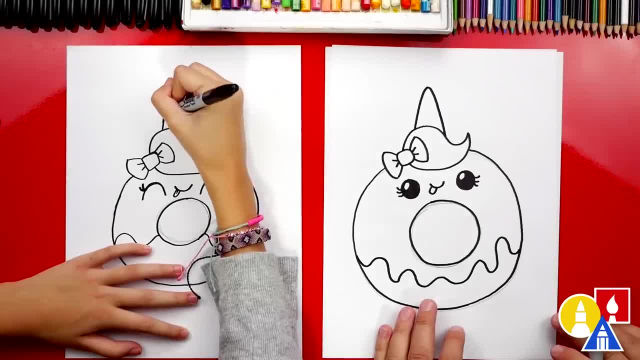 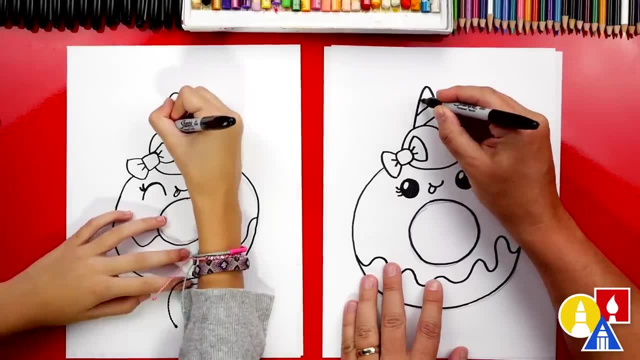 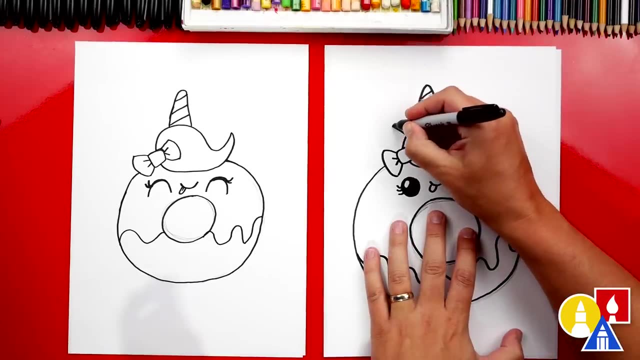 That's a friendly unicorn horn. Then we can also draw diagonal lines going across her unicorn horn. Now what should we add? The ears? Oh, that would make it even cuter. I'm going to draw another upside down V. This one's a little wider than the unicorn horn.